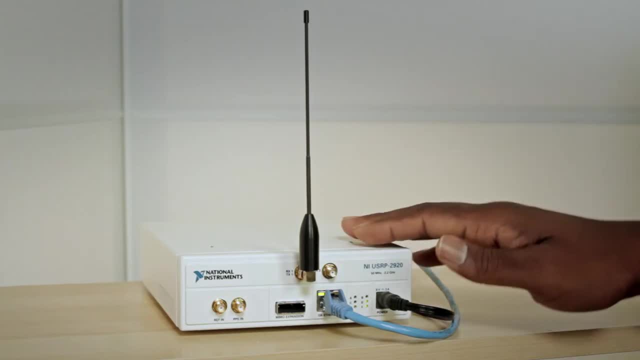 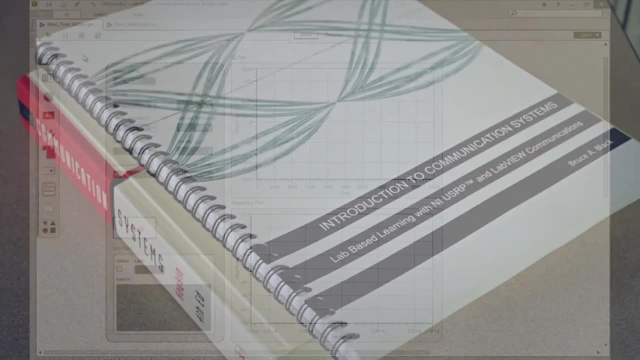 with real wireless signals. Here I have a USRP, a software-defined radio connected to my computer During a program that'll show some nearby radio stations. I'm going to be referring back to my communication systems textbook during the video In the book. an incoming 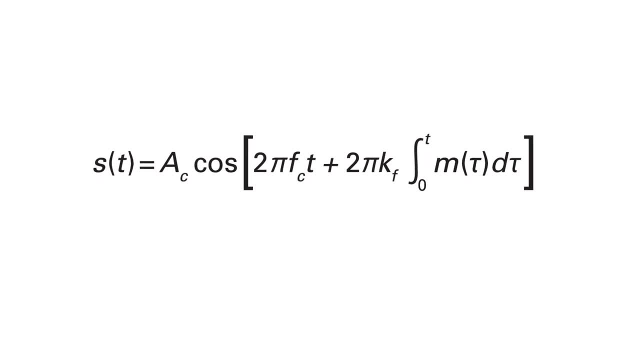 FM signal can be written as the equation shown We can see. our message is buried deep inside the formula. We can also represent the complex envelope of this signal as the equation shown. Here we have both magnitude and phase. Now our message is tucked away just inside the 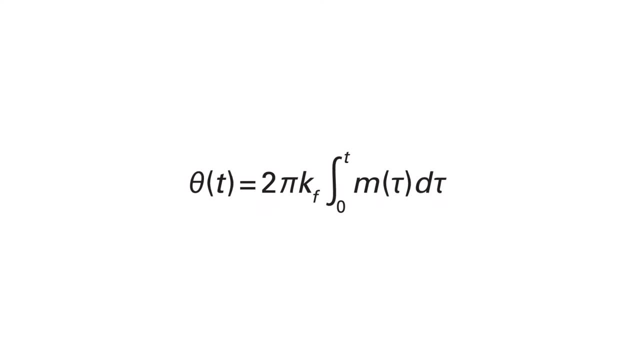 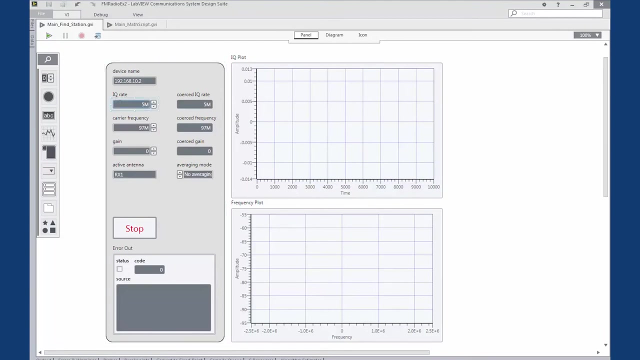 phase, but we can use arc tangent to get it. Lastly, we can take the first derivative to get the message signal. Let's see how software-defined radio can bring these equations to life. I'm first going to use this software-defined radio like a spectrum analyzer with a bandwidth. 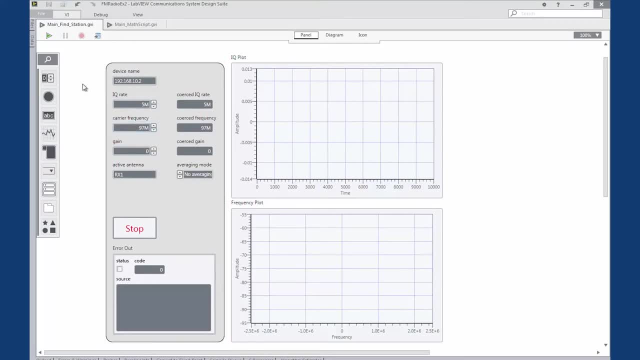 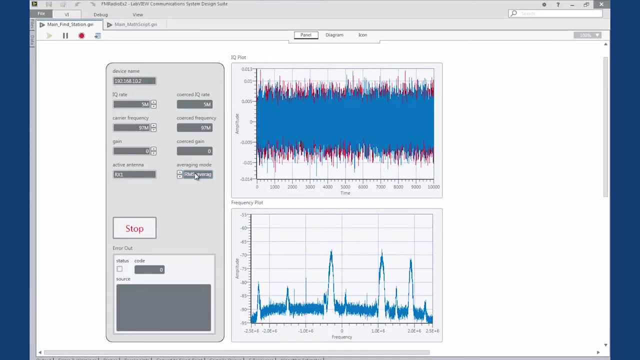 of 5 megahertz and a center frequency of 97 megahertz. In my frequency plot we can see some peaks. Now if we turn on averaging we can get a clear graph and we can see five, six and seven very strong signals coming through. These are the FM radio stations. 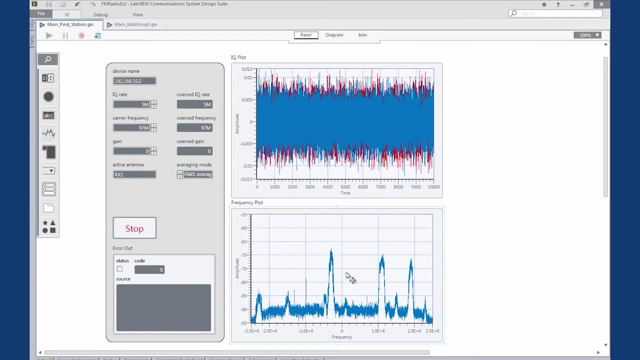 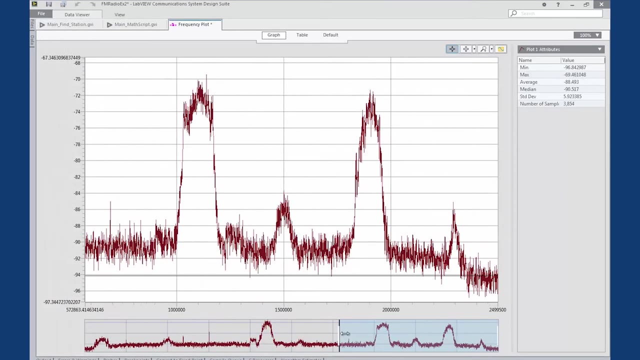 Students can see how nearby stations are separated, far enough that they don't interfere with each other. This is an important concept that relates to the bandwidth of each station. Students can further analyze these stations by capturing the graph data. Looking at the frequency plot, I can zoom in to just one of these stations. Alright, it looks like. 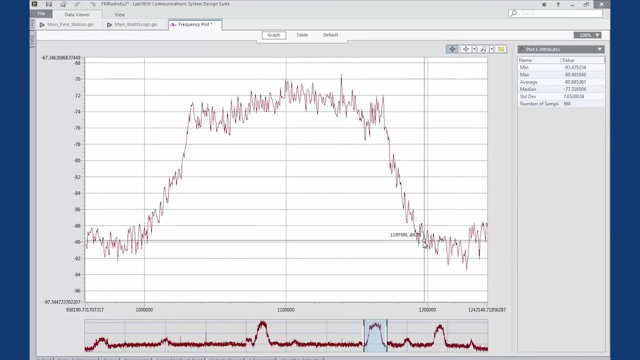 this signal has a bandwidth of not more than about 200 kilohertz. The maximum frequency deviation for broadcast FM is 75 kilohertz, and audio content is restricted below 20 kilohertz. A quick check via Carson's rule shows us that the maximum bandwidth should: 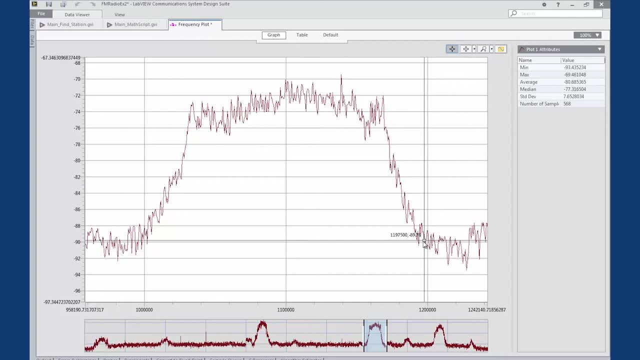 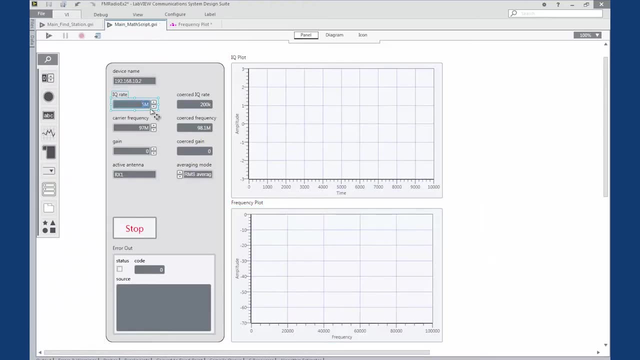 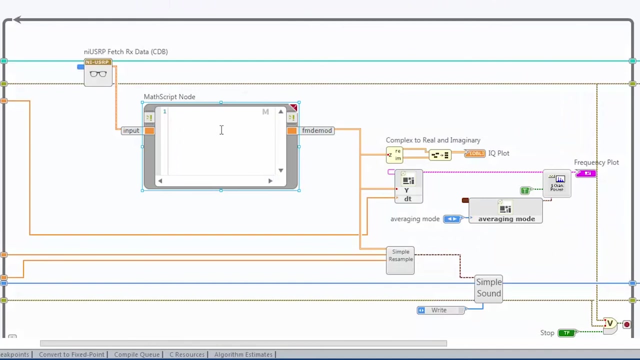 be about two times the sum of those numbers, or about 190 kilohertz. Perfect, I'll adjust my bandwidth to 200 kilohertz and adjust my center frequency up by about 1.1 megahertz. Now I'll be looking at the code. I can implement a little bit of math to demodulate.